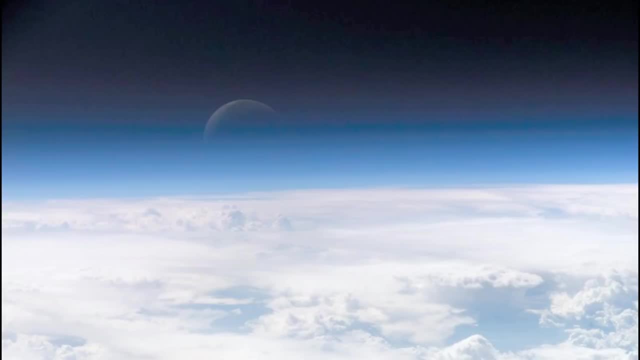 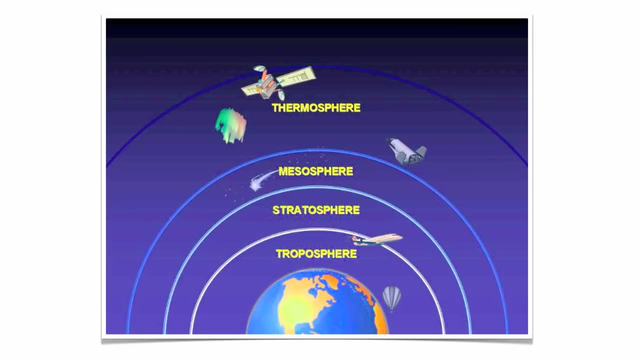 the white clouds. We're going to focus our attention on that layer where all the clouds are found. It's called the troposphere. We'll get to that in a second And as we increase our altitude or we increase our elevation above the earth, you're going to go from one layer to the 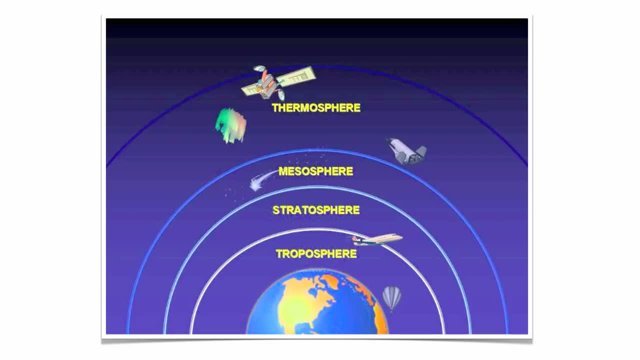 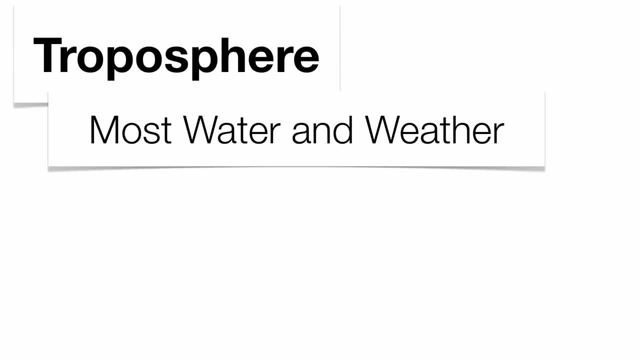 next Troposphere, stratosphere, mesosphere, thermosphere. So let's jump into the troposphere, talk a little bit about it. So, with this layer, it's going to be a layer that we currently live in. It's where the majority of our water vapor is found And, with that being said, that's where 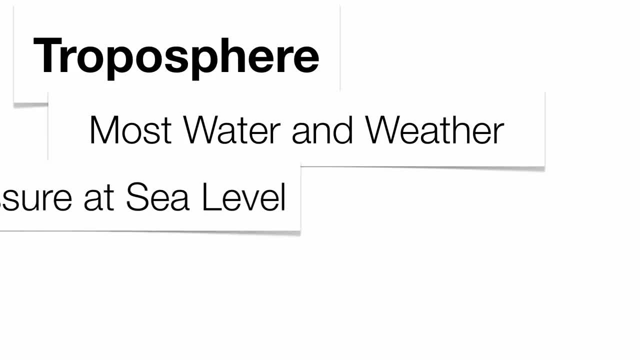 the majority of our weather is going to be found as well within our troposphere, Because we live, for the most part, close to sea level. we're going to have the majority of the troposphere, all the stratosphere, all the mesosphere. 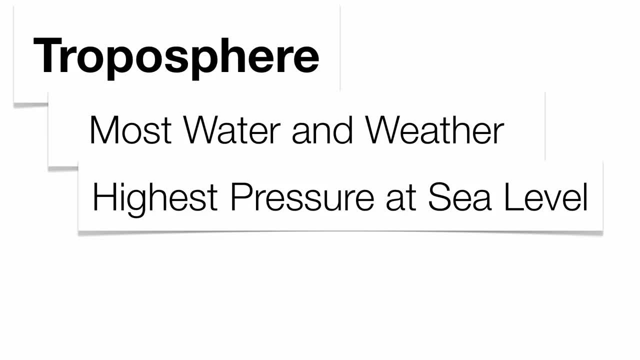 and all the thermosphere pushing down on top of us, So we're going to have the greatest atmospheric pressure found within the troposphere. As you travel up through the troposphere, you're physically getting further away from the earth, So temperature is going to decrease And that's evident when you 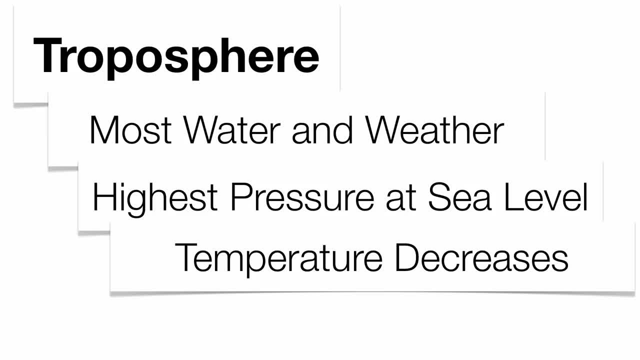 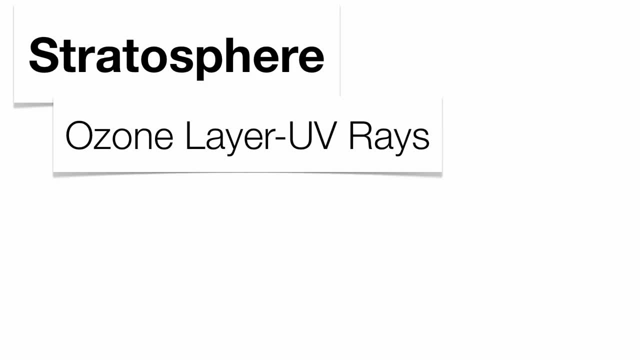 look at mountain ranges that are high enough. Many of them tend to be snow capped even in the summertime. Next layer up is what we call the stratosphere. Stratosphere is going to be super important to us because it's going to house what's called the ozone layer. The ozone layer is a part 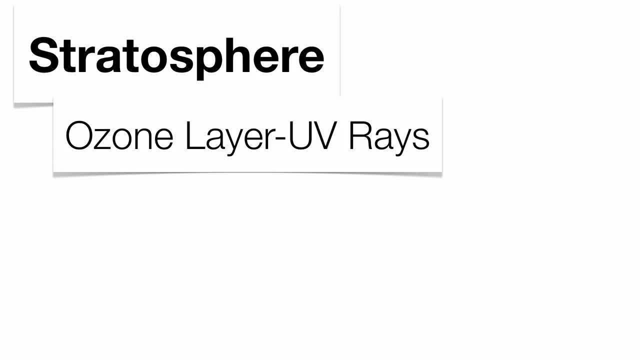 special part of the stratosphere that protects us from the sun. So we're going to have a lot of ultraviolet radiation from the sun, which is currently shortwave radiation, which scientists believe causes a high cases of skin cancer. Now, as you travel up through the stratosphere, 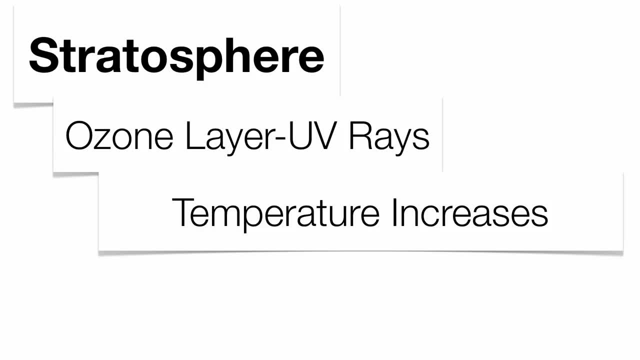 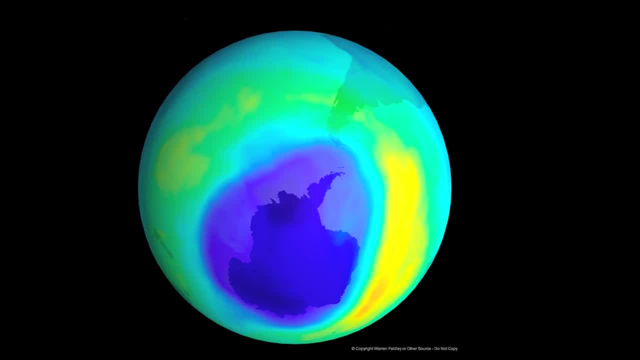 temperature actually goes up, Even though you're getting further away from the earth. it goes up because that ozone layer is absorbing a lot of the sun's energy, causing your temperature to go up. Now here's a picture of the ozone layer: the thinning of the ozone layer. A lot of people 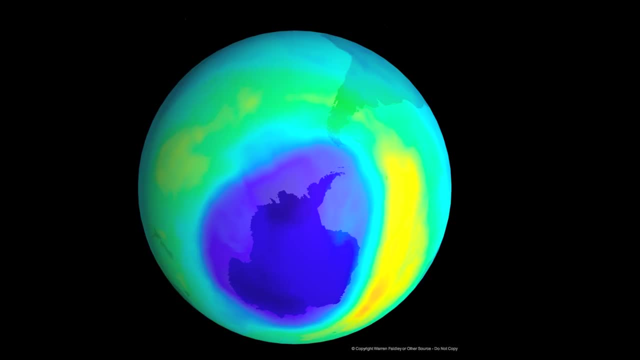 call it a hole, but it's actually a thinning of the ozone layer over top of Antarctica. Now, currently, CFCs, which are the CFCs, are the CFCs which are the CFCs, which are the CFCs which are. 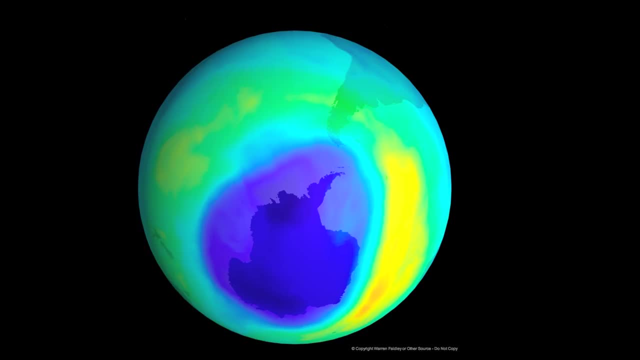 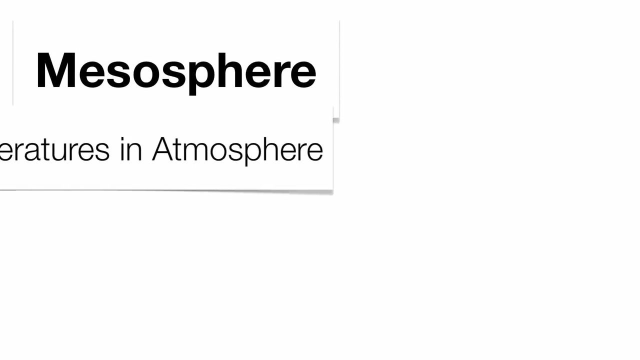 chlorofluorocarbons have attacked the ozone layer and have actually thinned it out over top of Antarctica. Since the banning of CFCs. the ozone layers actually start to repair itself. It's actually thickening over top of Antarctica. The next layer up is what we call the mesosphere. Now 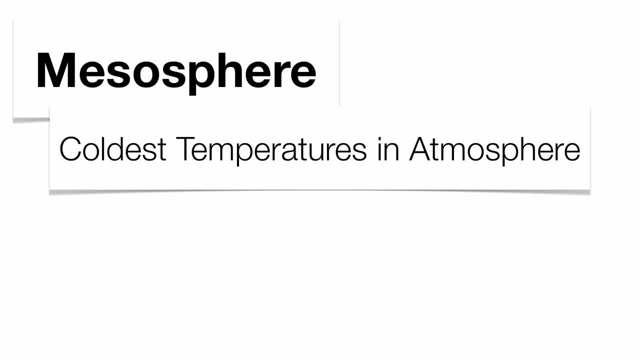 the mesosphere has some of the coldest temperatures in the atmosphere, And as you travel up through the mesosphere, temperatures drop dramatically, very simply because of the layer above it, which is called the thermosphere, And we'll talk about the thermosphere in a second. Okay, this is pretty. 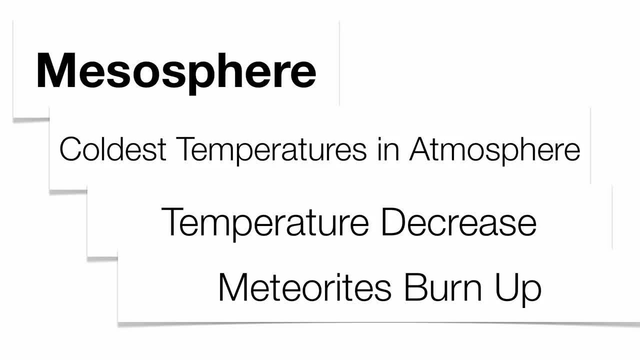 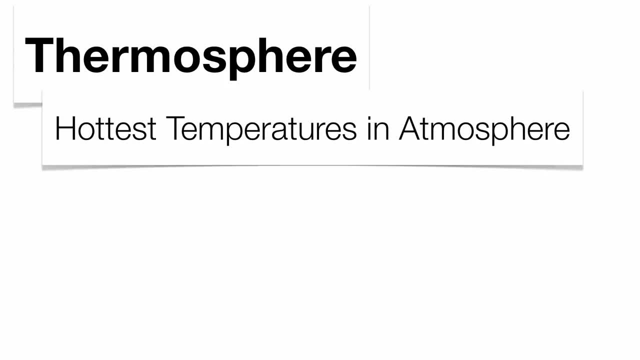 much where the layer where all your meteorites or your shooting stars are going to burn up as they enter our atmosphere. Now, the reason why the mesosphere is so cold is because the thermosphere is going to absorb a tremendous amount of the energy from the sun, gamma rays and x-rays. 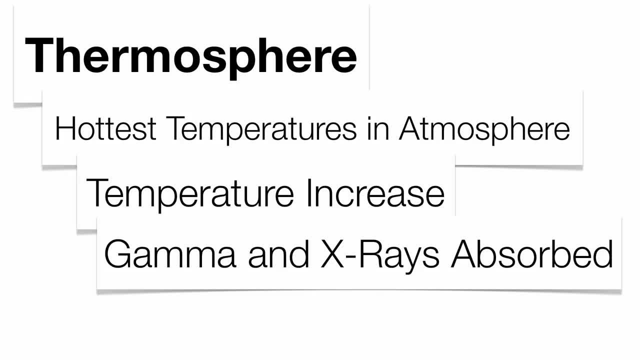 specifically those really nasty rays from the sun really really short wavelengths, really high frequency, very dangerous waves from the sun. They get absorbed by the thermosphere, So this tends to be some of the hottest temperatures in the atmosphere, because your temperature is going to go up through the absorbing of these rays And many times. 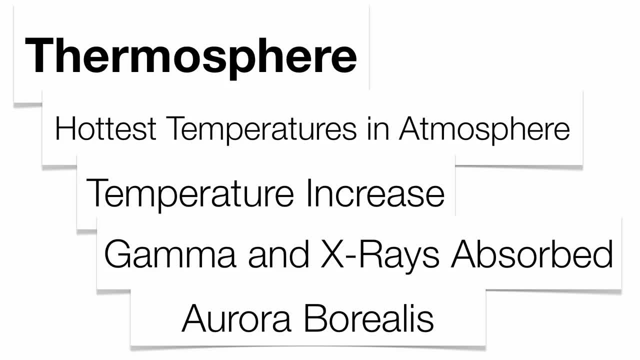 if you have an opportunity and you're lucky enough to see the Northern Lights or the Aurora Borealis or the Australis Borealis in the southern hemisphere, the southern lights- what will happen is those are going to be taking place in the thermosphere. So those are your. 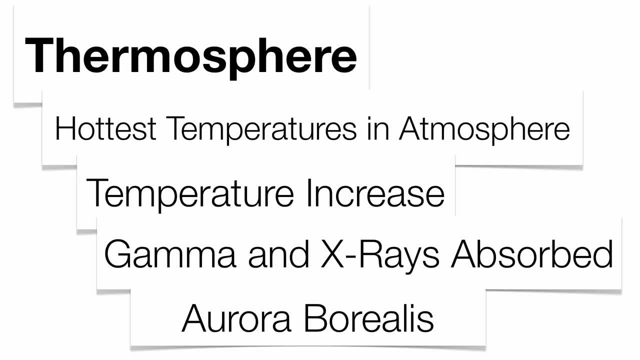 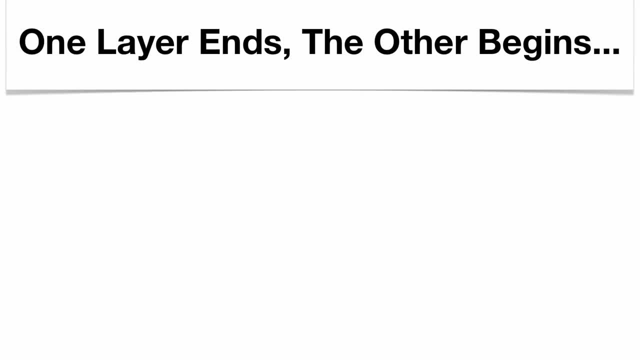 basically your four basic layers through the atmosphere. a couple of characteristics. you want a little bit more information about them. please go to wwwtheatmospherecom. Go to your reference table. Now, where one layer ends, the other one's going to begin. 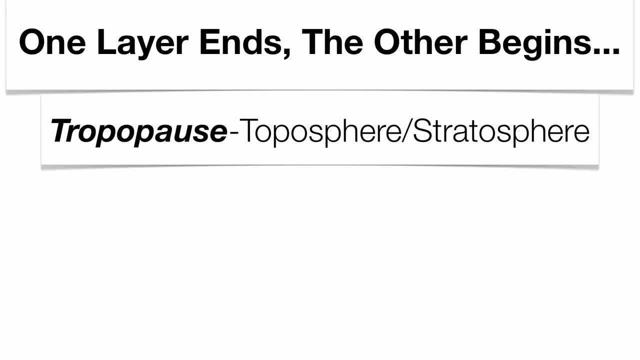 and it's all temperature dependent here. So where the troposphere ends and the stratosphere begins, that's what we call the tropopause. You get a very, very distinct boundary in temperature differences between the stratosphere and the troposphere. there So the boundary. between those two layers is what we call the tropopause. Where the stratosphere ends and the mesosphere begins is what we call the stratopause, And where the mesosphere ends and the thermosphere begins, that's what we call the mesopause. Okay, so make sure you. 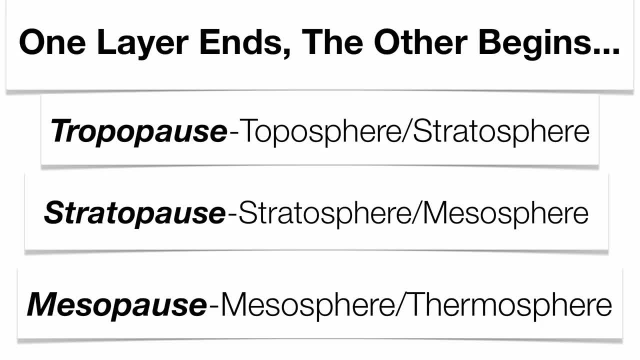 know the difference between the spheres, which are the layers of the atmosphere, and the pauses, which are the breaks. Now, where one layer ends and the other begins, is all temperature dependent? If you go to your reference table, you'll see that relationship. Now you do. 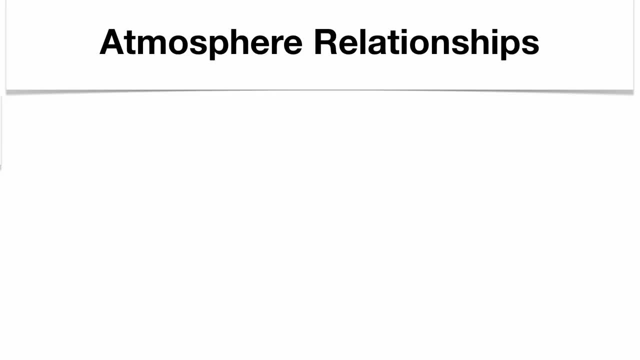 have a couple atmospheric relationships with the increase in altitude above the surface. So water vapor, because water vapor is solely concentrated for the most part in the troposphere- as you increase your altitude, as you go up through the atmosphere, water vapor content is going to decrease.